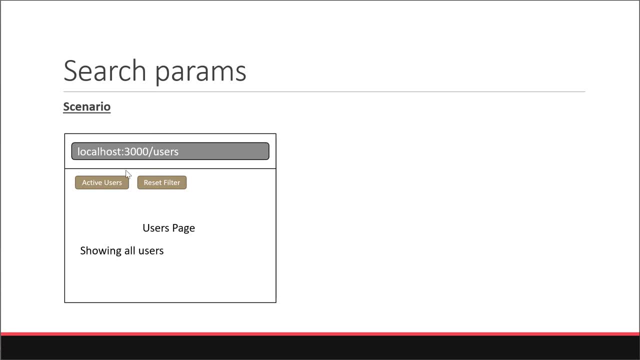 page. let's add two buttons: one that says active users and one that says reset filter. By default, the page renders the text showing all users On click of active users. we're going to add a search param called filter and set it to. 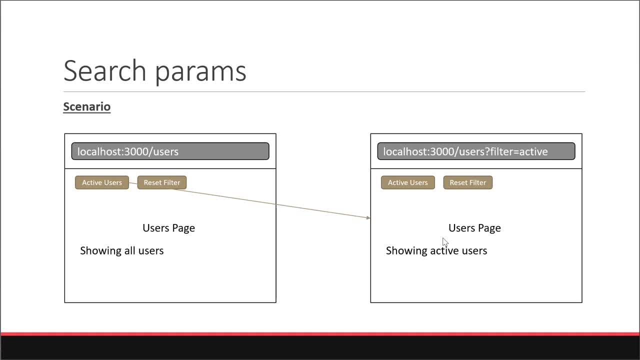 active In the component, we will display text showing active users. If you click on reset, we remove the filter search param and revert the text. Changing the text is pretty simple and your app might have more complex requirements. I just want to ensure you understand the concept of search params and how to put it to use. 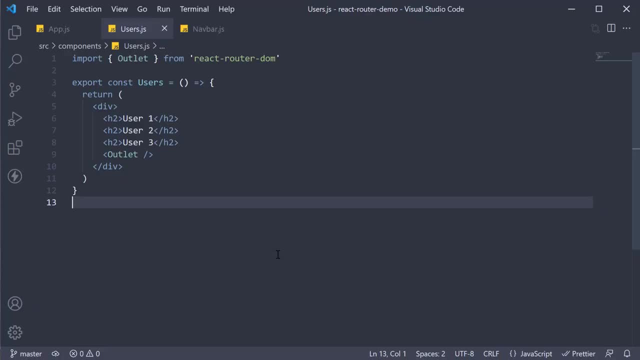 is up to you, Let's begin. Let's begin For step one. in the users component, let's add two buttons: Active users and the second button is reset filter. For step two, on click of these buttons, we need to add or remove the search param. 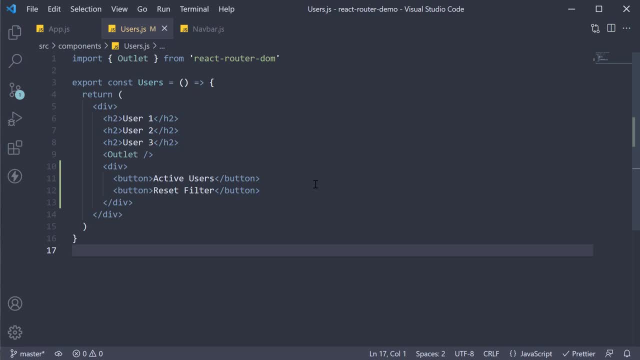 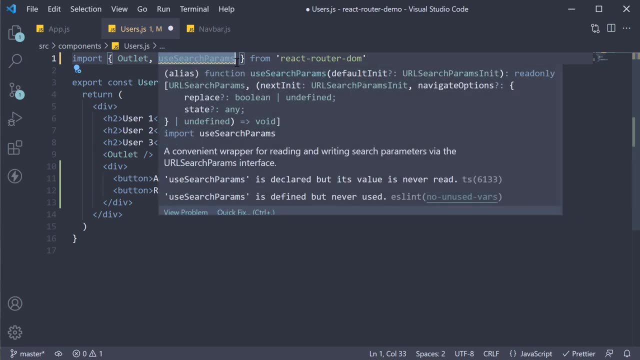 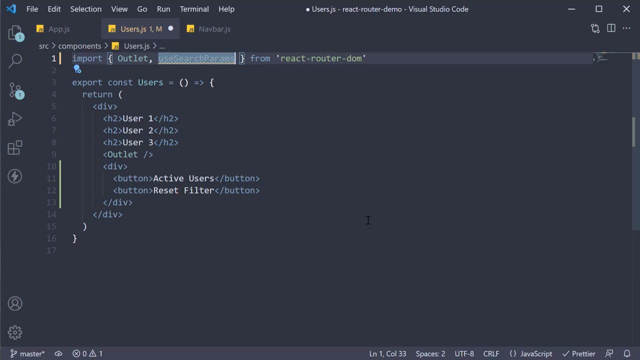 To deal with search params, React Router provides a hook called use search params. Import it at the top. This hook behaves similar to the use state hook in React. Instead of storing state in memory, though, it is stored in the URL Within the component invoke the hook. 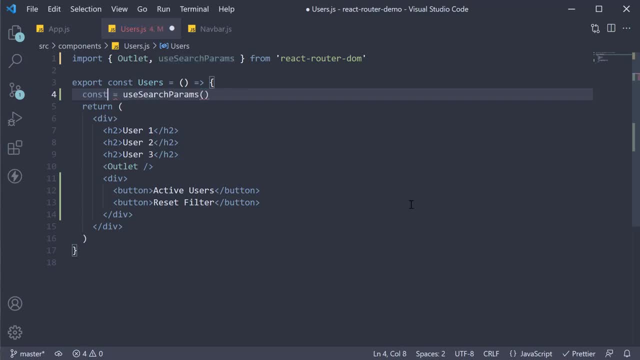 Use search params. The hook returns two values, of which the first one is an object which we are going to call as search params. The second value returned is a function to set the search params. Let's call this setSearchParams. As you can see, it is very similar to use state. 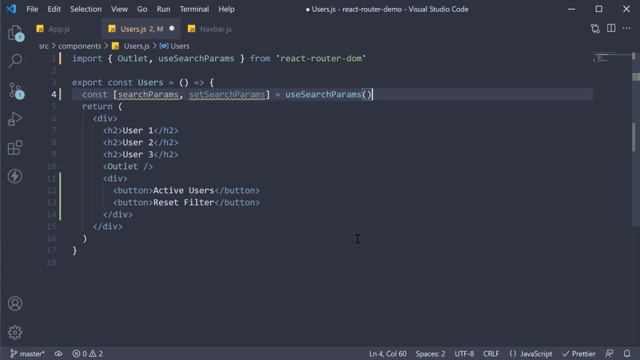 Now, using setSearchParams function, we can add or remove the parameter First on click of active users button. On click, We're going to have an arrow function where we call setSearchParams And we pass in an object with one property called filter, whose value is active. 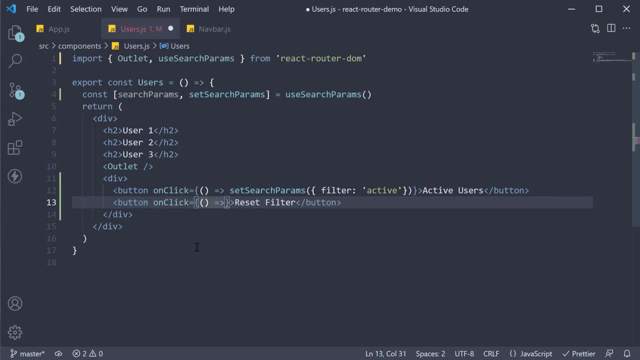 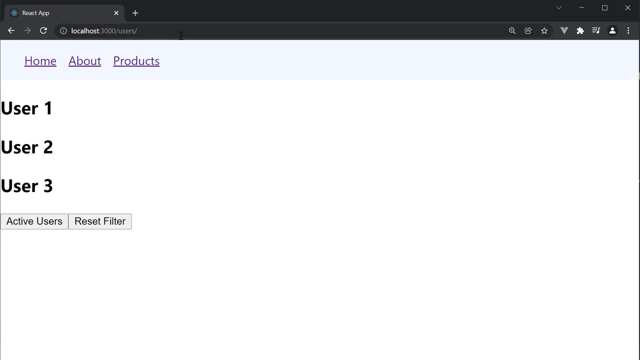 Next, on click of resetFilter button, we call setSearchParams again, but this time with an empty object. Let's save the file and test if this works. So we are done. So we are here at localhost: 3000 slash users. I click on active users. 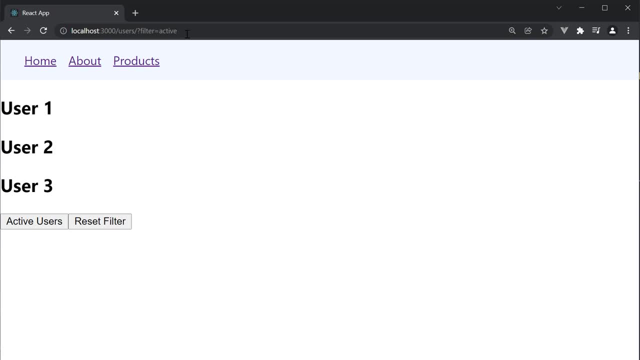 And you can see we have question mark. filter is equal to active. Click on resetFilter And the search param is removed. Now what we need to do is check if filter search param is set to active and display the appropriate text. So for step three, 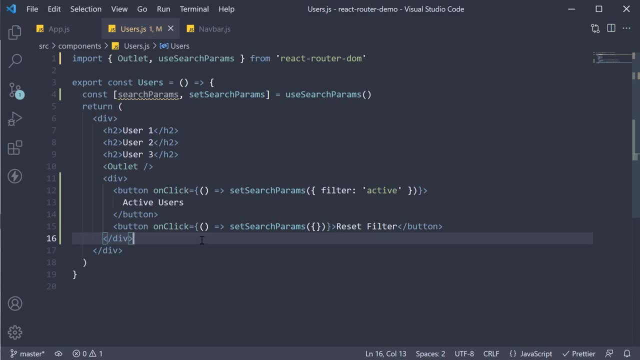 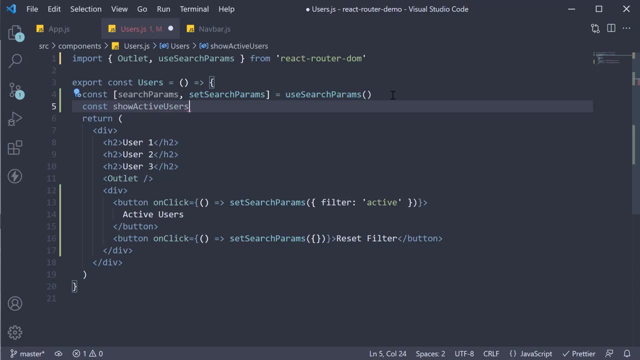 For component. we make a check on the filter parameter. Const show active users And this is going to be a boolean value. To get hold of the filter parameter, we use the get function on search params. So search params dot get. What is the param name? 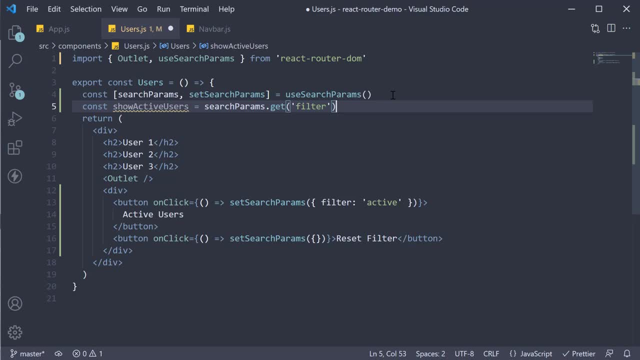 It is filter. We then compare the value with the string String active. So show active users is true if we click on active users button and false if we click on resetFilter button. Let's use it to render the JSX Curly braces. 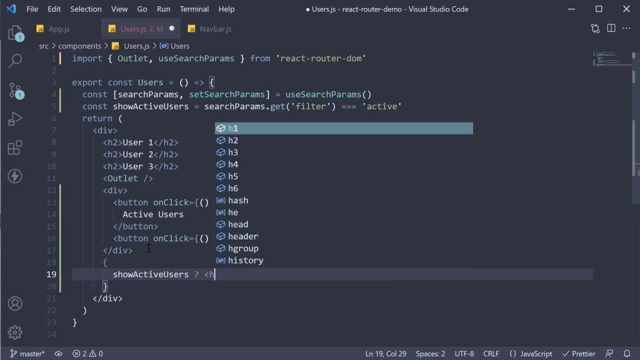 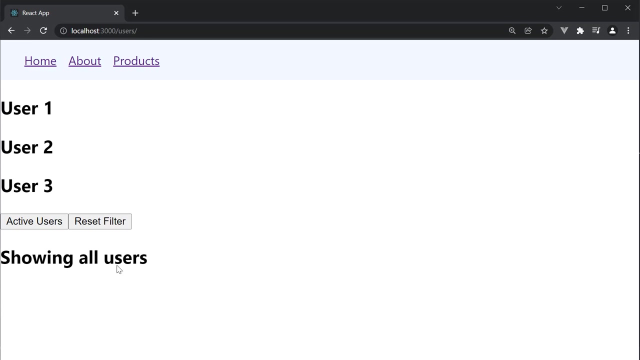 Show active users. if it is true, Return an h2 tag that says showing active users, And if it is false, Return an h2 tag that says showing all users. If we now take a look at the browser, You can see the text showing all users. 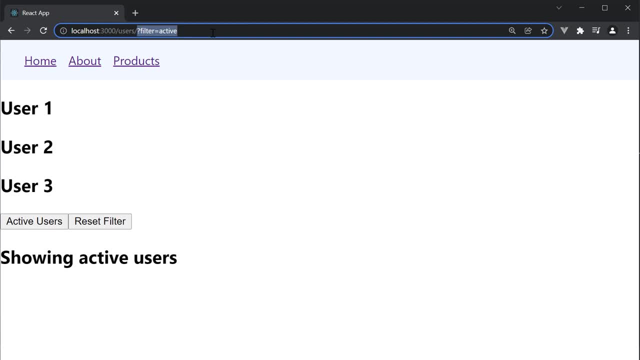 Click on active users. We see the search param in the URL And the text is now showing active users. Reset filter, Showing all users once again. Our code with search params is working as expected. Using search params is pretty common when you have to apply filters in a listing page.